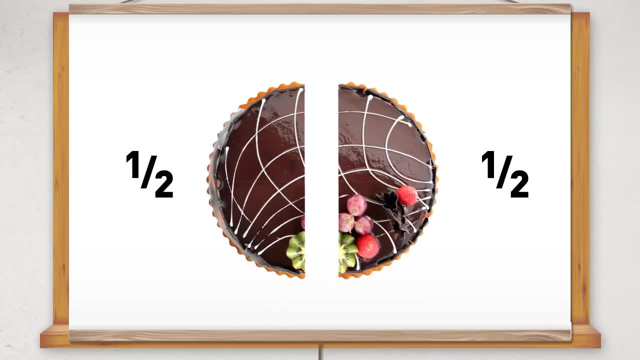 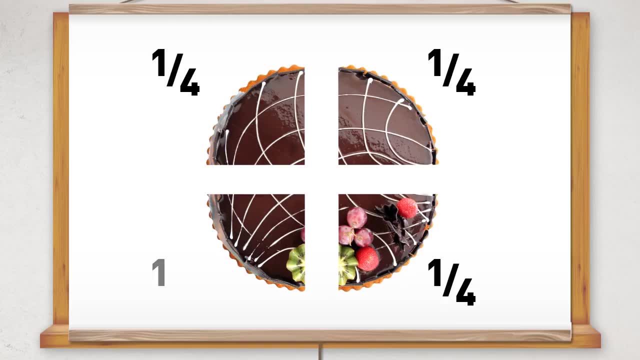 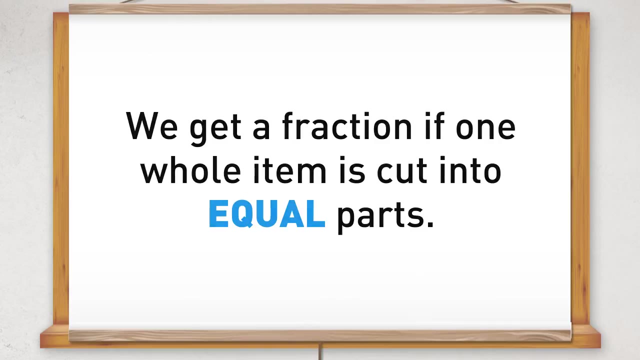 half a cake on one side and half a cake on the other. If it was cut into four equal pieces, each piece would be one quarter of the cake. We get a fraction if one whole item is cut into equal parts. For example, this pizza has been cut into eight equal parts, So each. 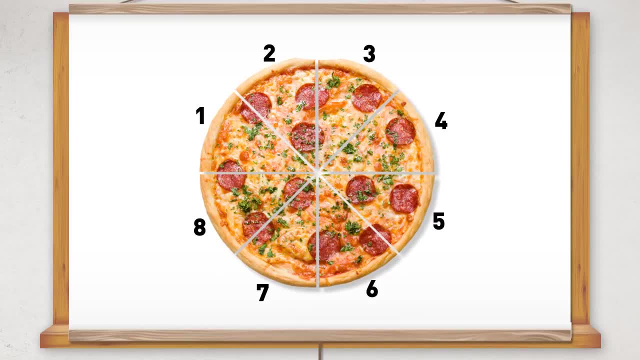 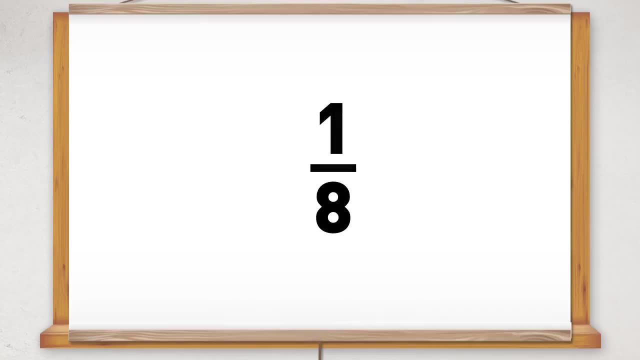 piece is one eighth of the pizza. To write it in figures, we write a one on the top of the fraction and an 8 on the bottom. The top number of the fraction is called the numerator. The bottom number is called the denominator. If the top number is a 1, the 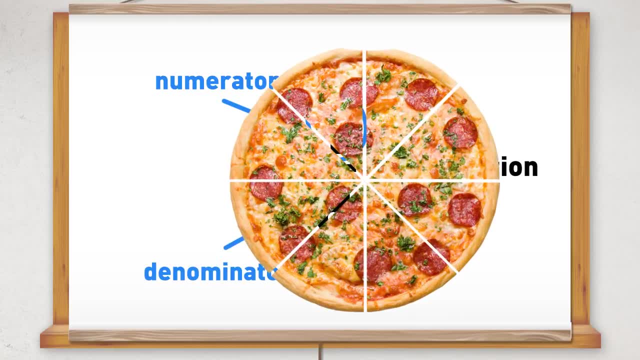 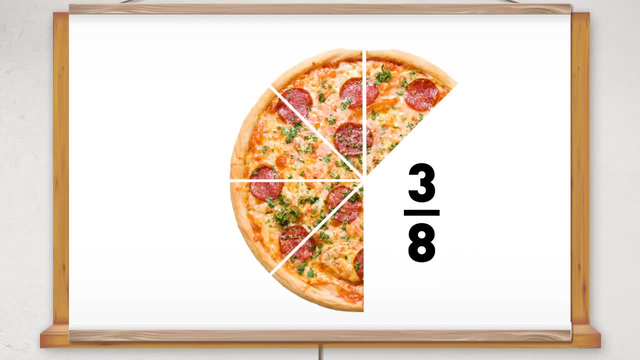 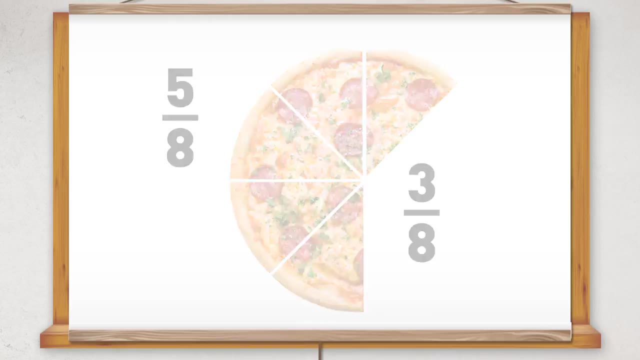 fraction is called a unit fraction. If I had eaten three parts of the pizza, I would have eaten three-eighths of the pizza. I would then have five pieces left over, So five-eighths of the pizza would be remaining If a whole item is divided into two equal parts each. 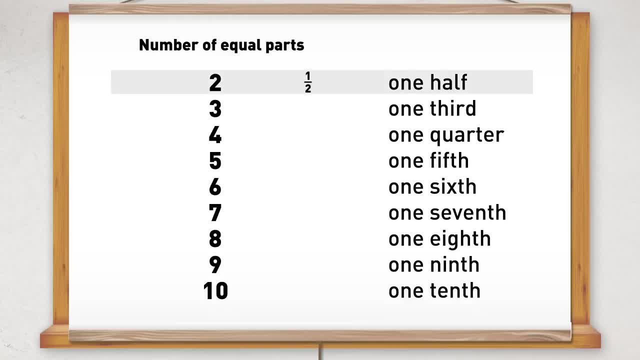 part would be one out of two parts. one-half. If a whole item is divided into three equal parts, each part would be one out of three parts. one-third. If a whole item is divided into four equal parts, each part would be one out of four parts. one-quarter. If a whole 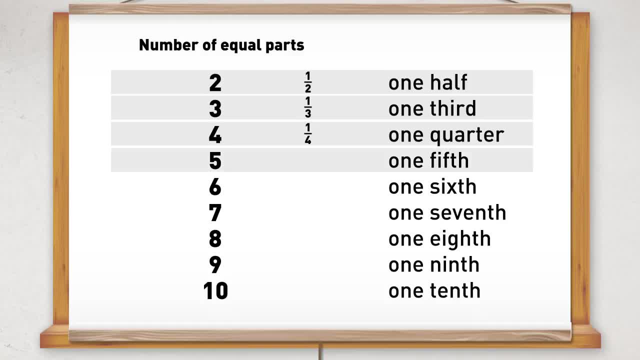 item is divided into four equal parts, each part would be one out of four parts. one-quarter: If a whole item is divided into 5 equal parts, each part would be 1 out of 5 parts 1. fifth, If a whole item is divided into 6 equal parts, each part would be 1 out of 6 parts 1. sixth. 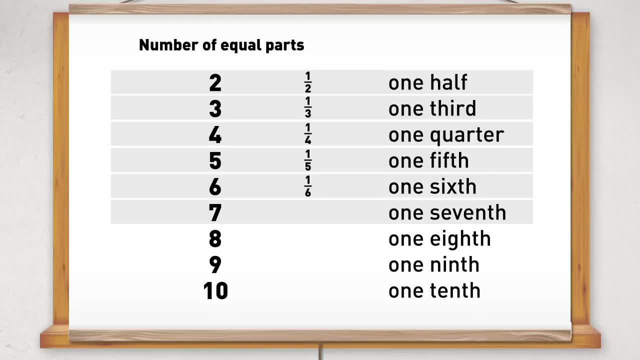 If a whole item is divided into 7 equal parts, each part would be 1 out of 7 parts, 1. seventh. If a whole item is divided into 8 equal parts, each part would be 1 out of 8 parts, 1. eighth. 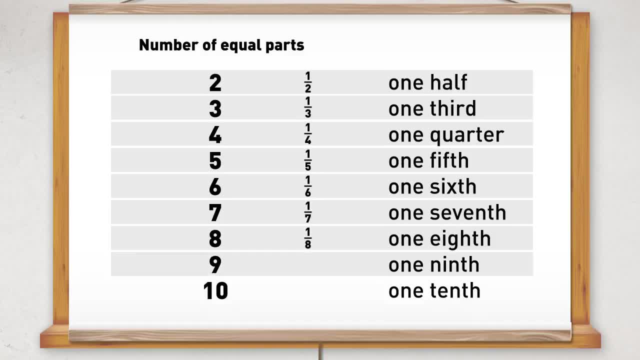 If a whole item is divided into nine equal parts, each part will be one out of nine parts one-ninth. If a whole item is divided into ten equal parts, each part will be one out of ten parts. one-tenth.